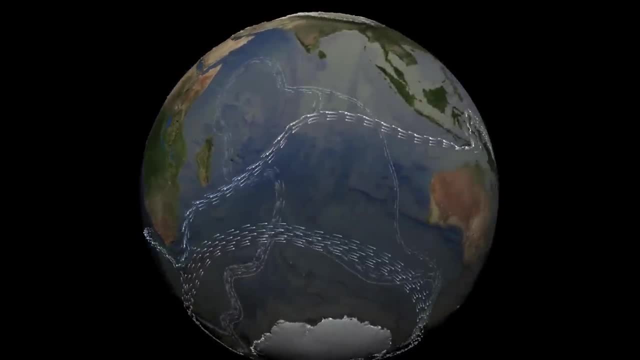 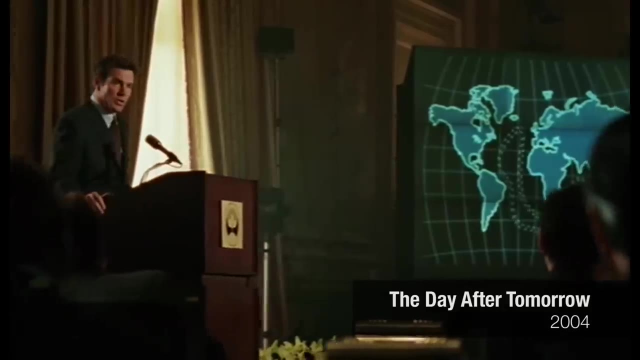 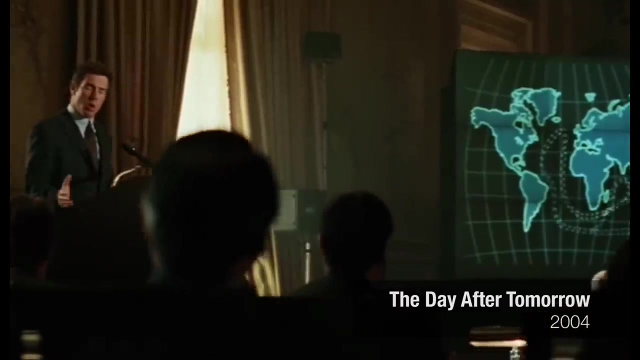 that global conveyor belt, that so-called thermohaline circulation, popularized, of course, in the film The Day After Tomorrow. The Northern Hemisphere owes its temperate climate to the North Atlantic. current Heat from the sun arises, It thrives at the equator and is carried north by the ocean. 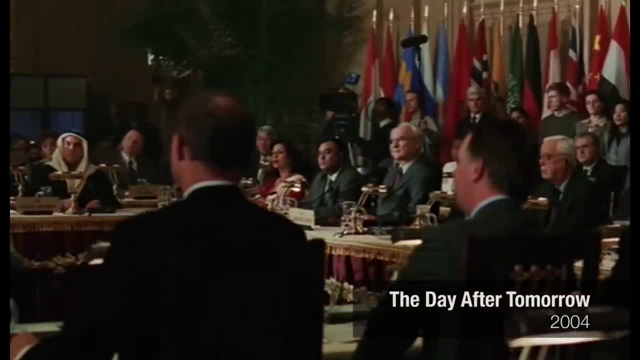 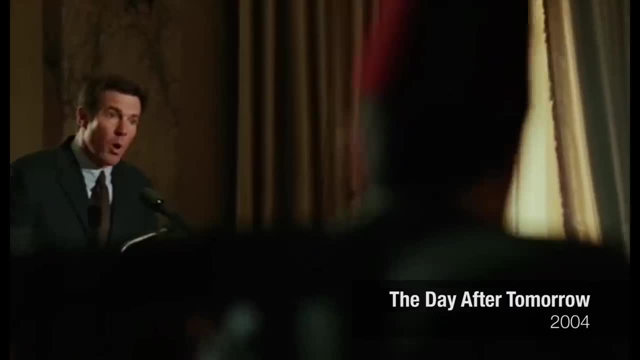 But global warming is melting the polar ice caps and disrupting this flow. Eventually it will shut down and when that occurs, there goes our warm climate The Day After Tomorrow. the film: the premise is based on science, but it was greatly overblown. 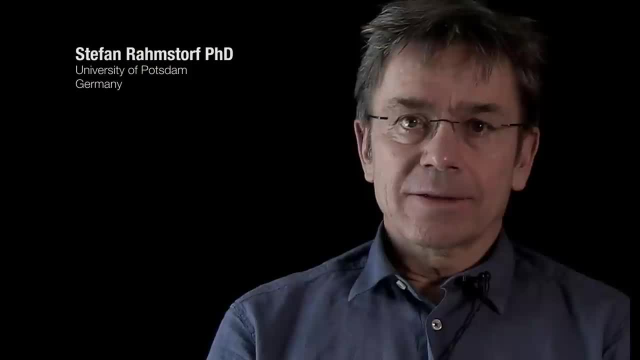 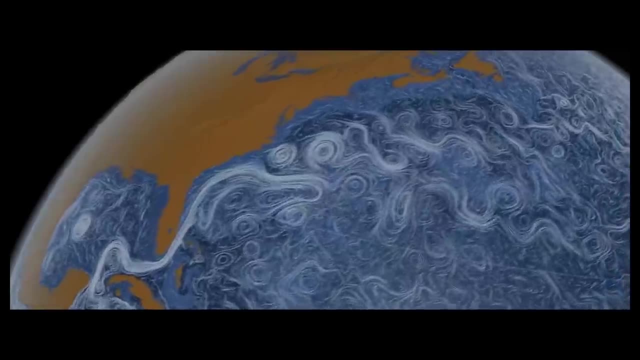 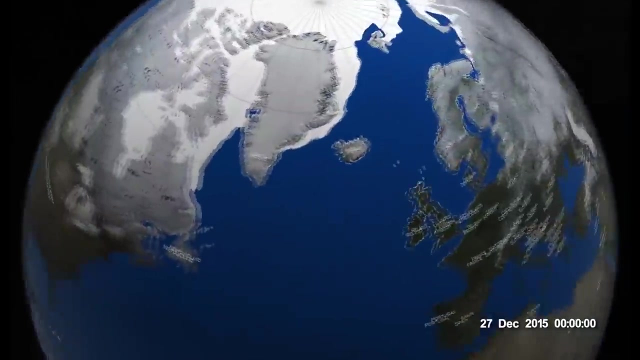 And frustrated a lot of climatologists. The Gulf Stream system is a very important part of the climate machinery of our planet because it transports huge amounts of heat and is the reason why the whole region around the Northern Atlantic is warmer by several degrees centigrade. 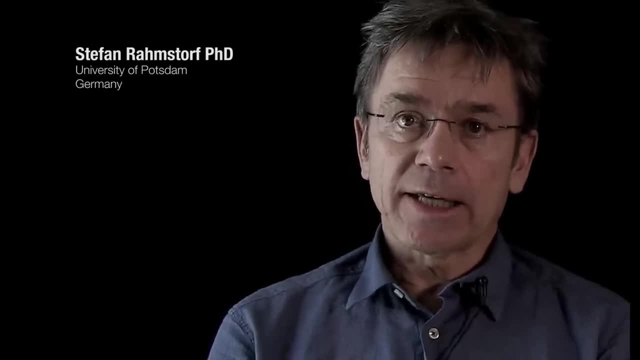 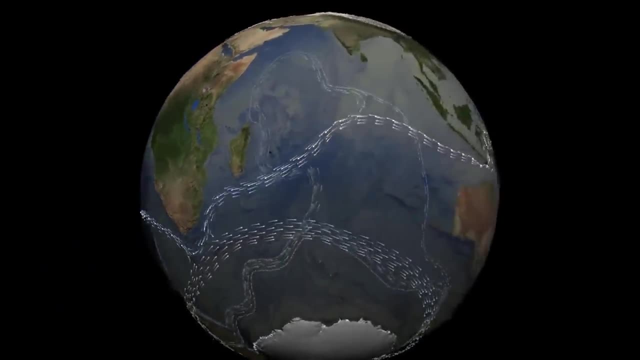 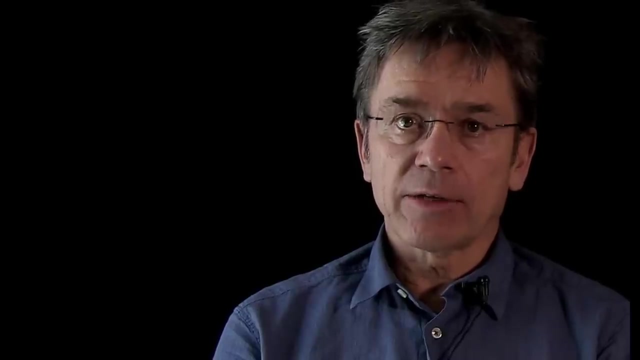 compared to what would be normal on that latitude. There has been a concern since the 1980s that this system might be unstable and that it's not going to work. Due to the global warming, we are actually slowing down the Gulf Stream system. 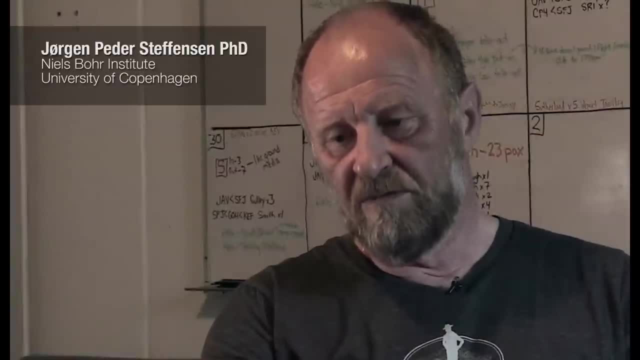 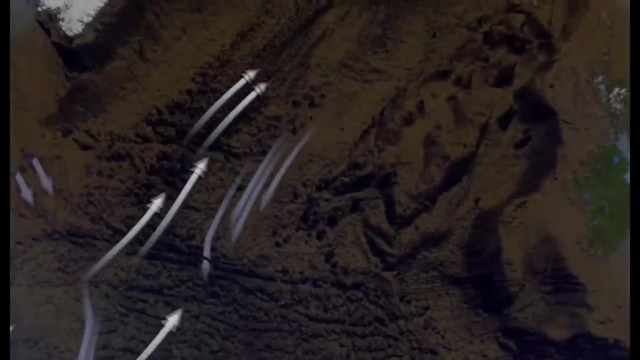 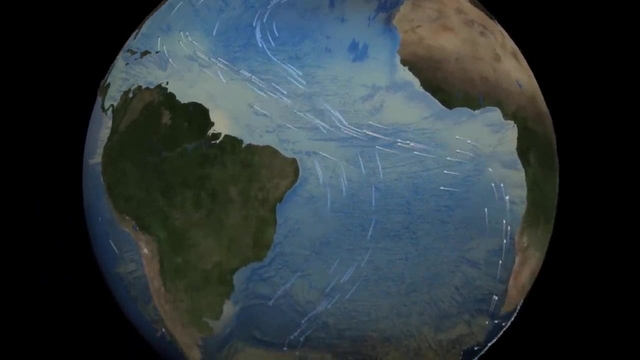 What if what we do now is introducing so much fresh water into the North Atlantic that the North Atlantic current would sort of stop? That would make it terribly cold in Denmark, where I come from, because all of Northern Europe is placed at completely unreasonable latitudes. 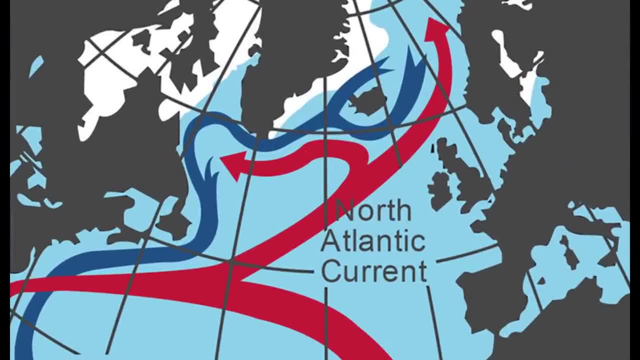 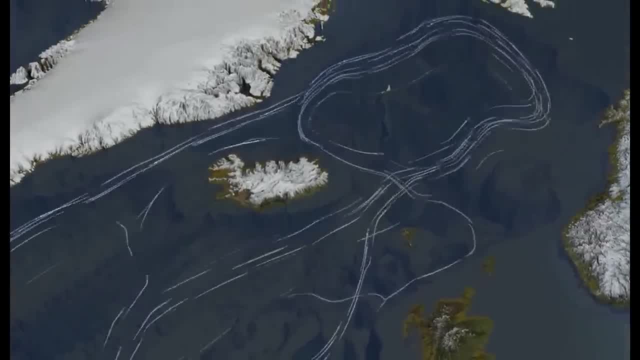 Just because we have the North Atlantic current, we have remote heating, so to say. If that's going to be switched off, we're getting very, very cold, But still the Earth could get warmer on average. It's just a distribution problem now. 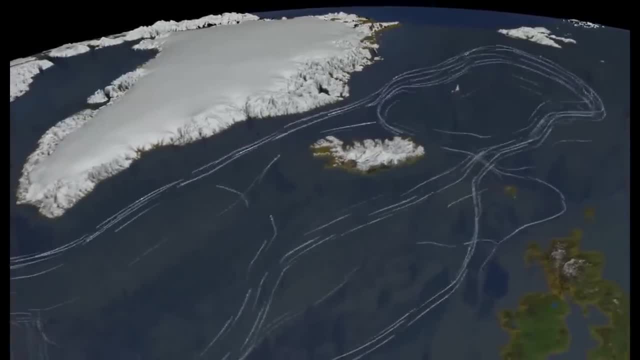 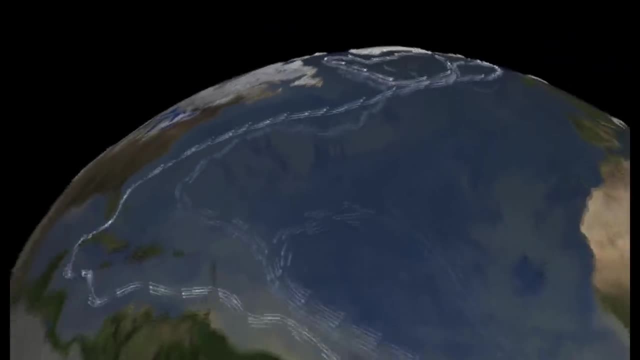 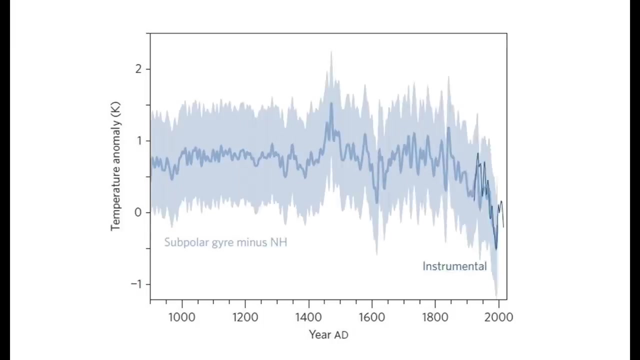 In principle, there's no reason why the Earth could not get warmer, but still Northern Europe and North America could get cold. Still that area is not large compared to the global area. We are 50 years to 100 years old, 50 years to 100 years ahead of schedule. 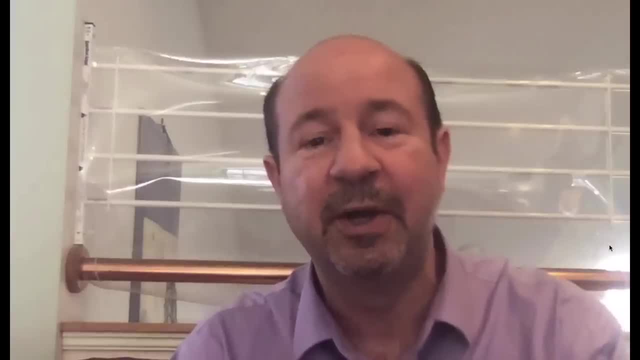 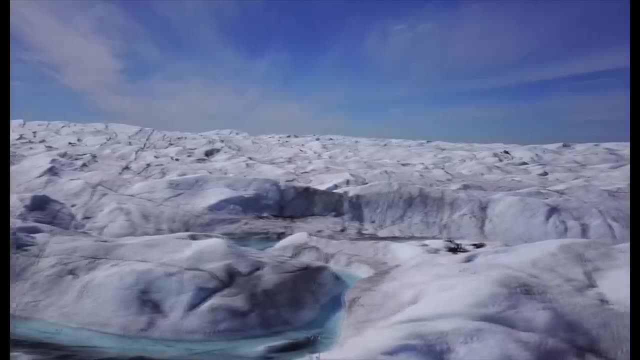 with the slowdown of this ocean circulation pattern relative to what the models predict. Why might that be true? Well, one of the things that the models also aren't capturing is the rate at which we are losing ice from the ice sheets: the West Antarctic ice sheet and the Greenland ice sheet.